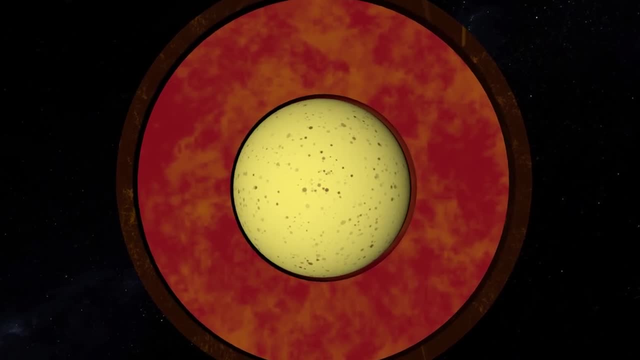 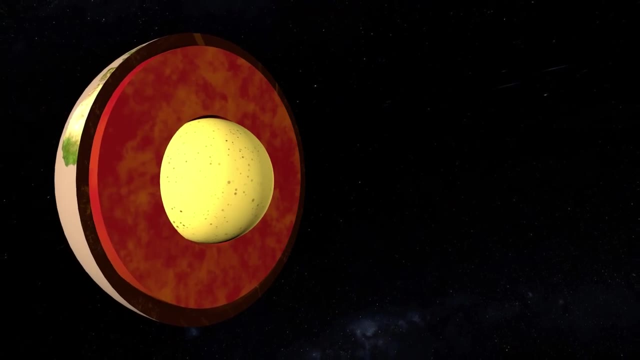 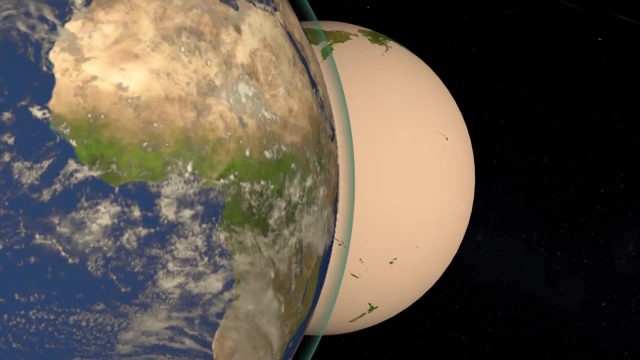 magma and sand. The closer we get to the inner core, temperature density and pressure progressively increase. The geosphere is made up of three concentric layers: the crust, the mantle and the core. The crust is the thinnest outermost layer of the geosphere. The thickness of the 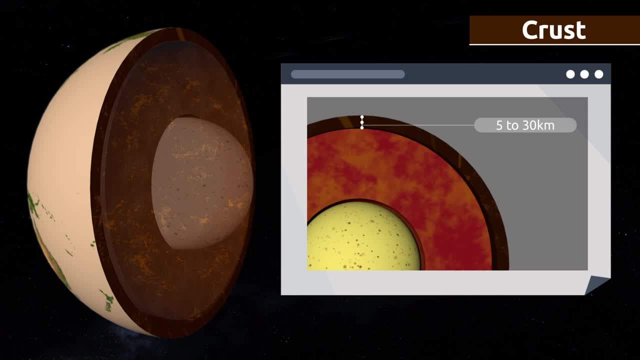 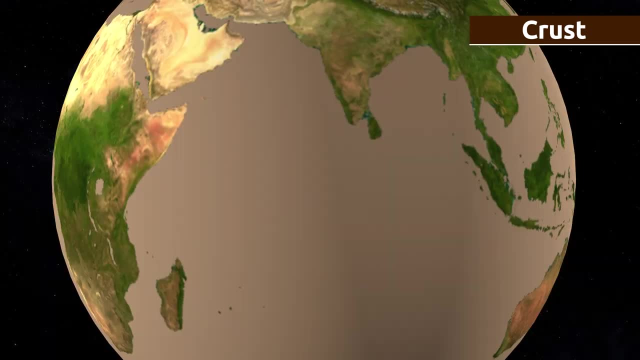 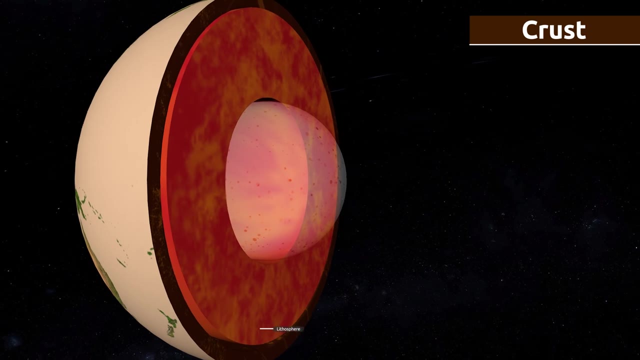 crust varies from 5 to 30 kilometers, depending on where you are on the Earth. The crust is made up of continents and the bottoms of the oceans. The geosphere is broken up into several tectonic plates. These make up the crust and also the mantle, and they are found in a layer. 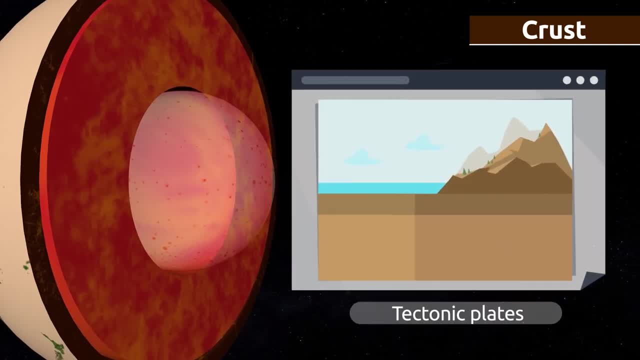 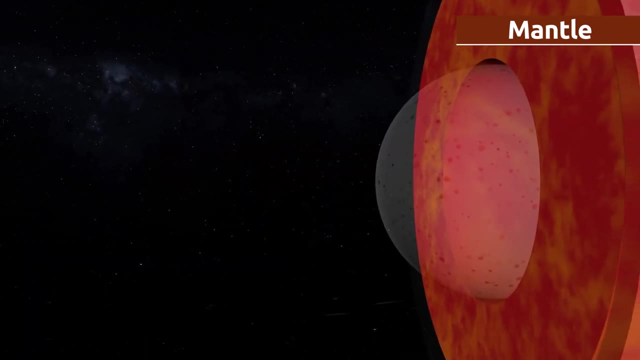 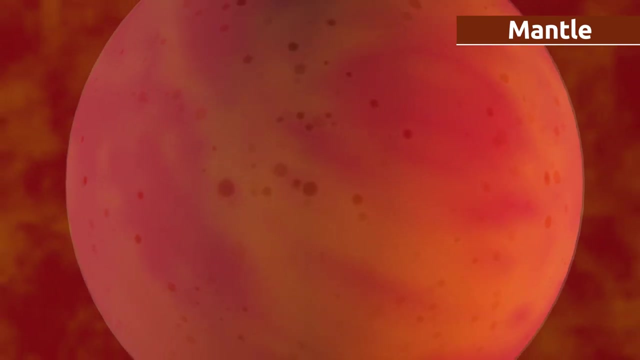 called the lithosphere. Tectonic plates are constantly moving, molding the crust. Their movements causes earthquakes. The second layer of the geosphere is called the mantle. It is 82% of the Earth's volume, being 2,900 kilometers thick. The temperature of the mantle is really high, ranging from 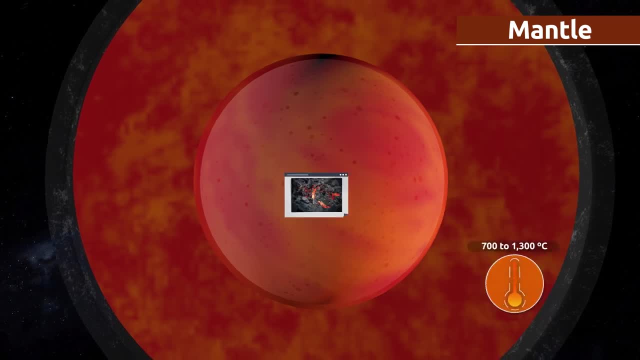 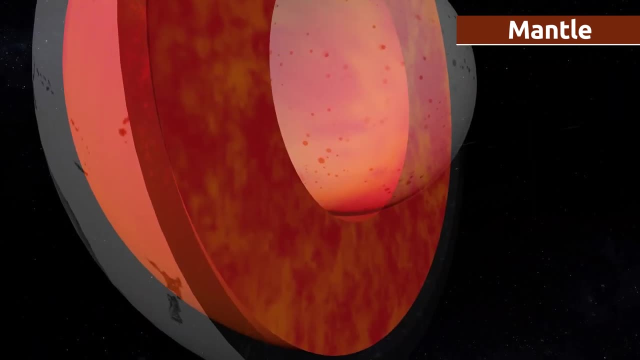 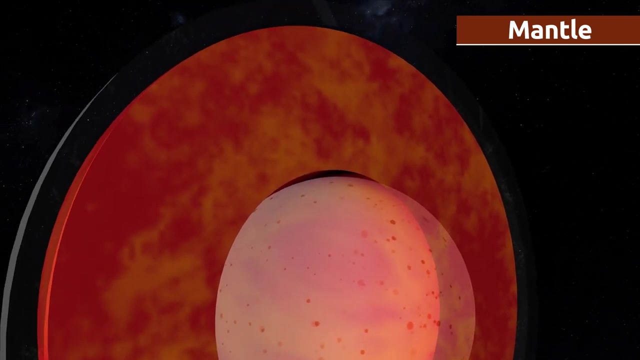 700 to 1,300 degrees Celsius. That's why it's made up of molten rock called magma. Sometimes, magma finds its way up to the surface and flows up through the mantle. Magma is also made up of the geosphere. The crust is the thinnest outermost layer of the Earth. The 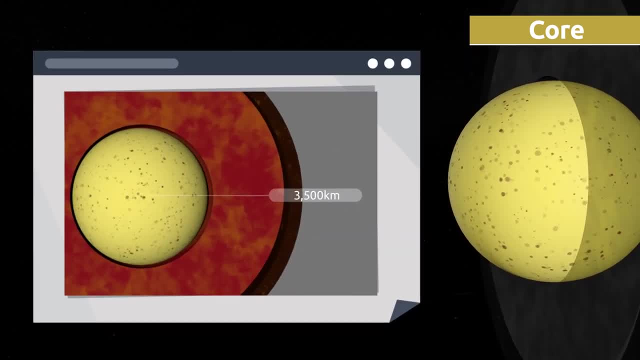 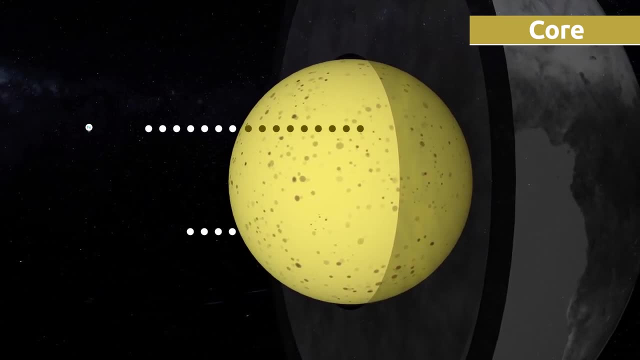 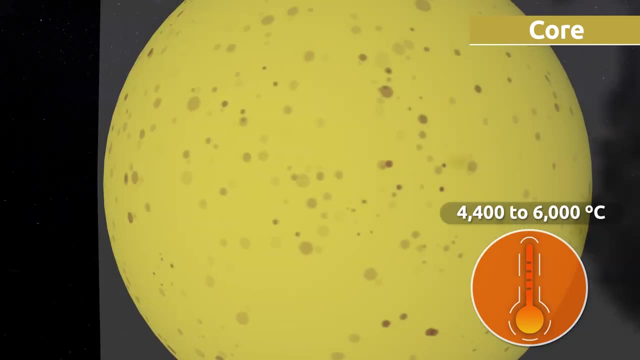 crust is made up of 3,500 kilometers thick. The inner part of the core is made up of solid iron, where the outer part is made up of liquid iron and nickel. The temperature in the core is ultra high, ranging from 4,400 to 6,000 degrees Celsius. The wide ranges of temperature 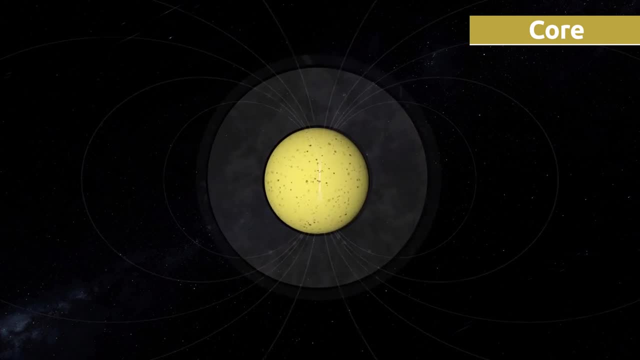 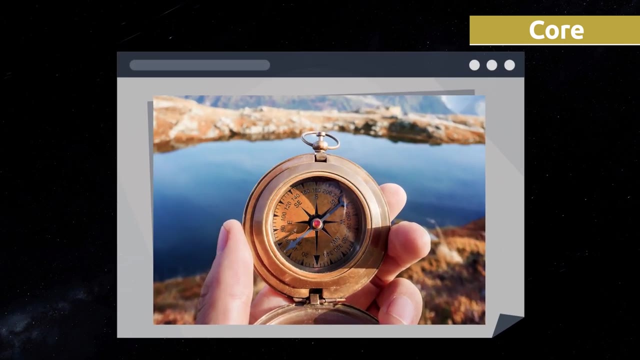 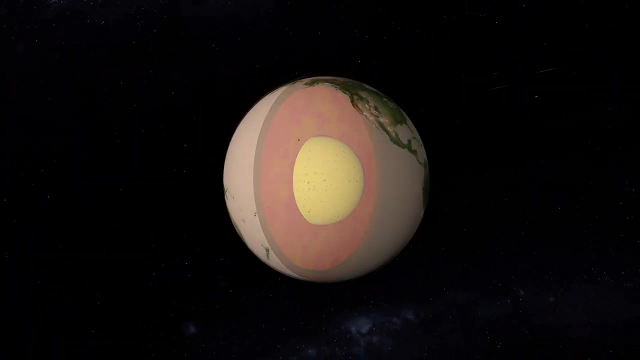 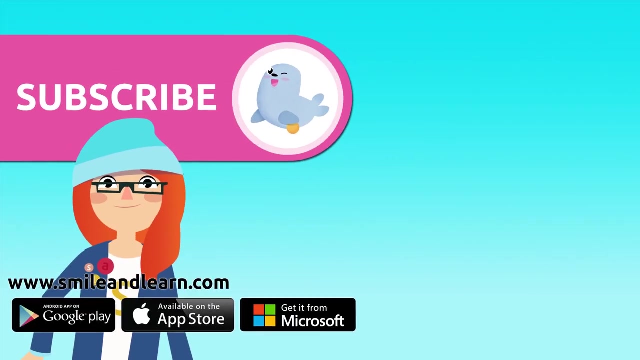 and pressure conditions in the outer core cause the molten metal to move. This results in the formation of electric currents that produce magnetic fields. Did you know that, thanks to these magnetic fields, we are able to use instruments like the compass? These are the layers of the geosphere. Did you like learning about them? 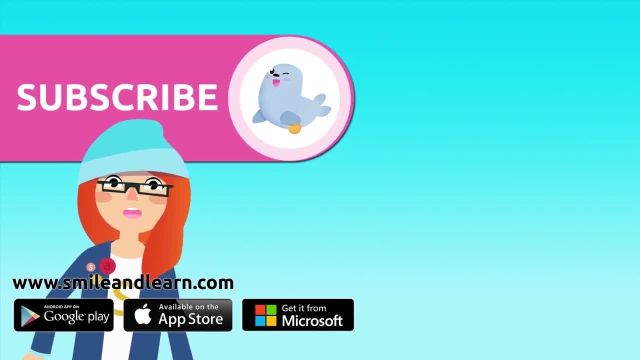 Did you like the video? We have so many more. Subscribe by clicking on the seal Ah, and if you want to keep watching more videos, click on the boxes.